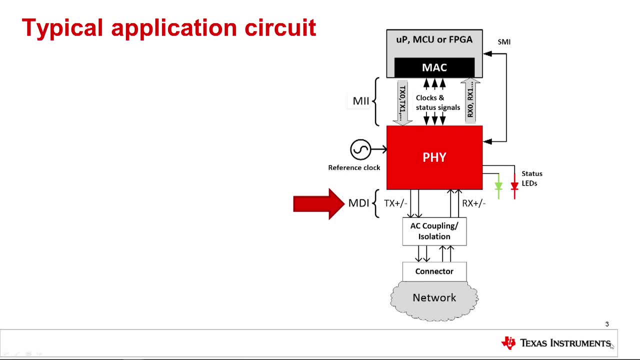 Unlike the MII, the signaling characteristics of the MDI depends on the nature of the physical channel, which could be either copper or fiber. The PHI usually provides general-purpose input-output pins or GPIO, which typically can be used to either drive status LEDs. 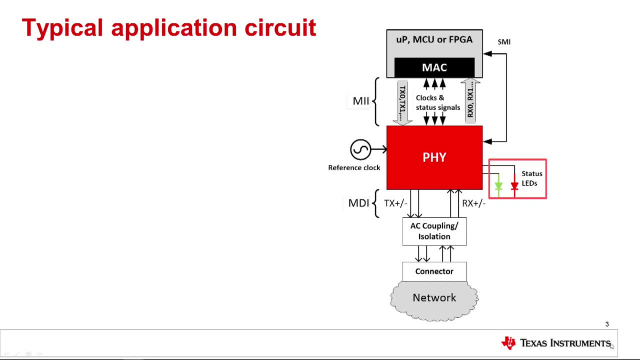 or to provide access to other internal signals. When used as LED drivers, they can give you visual indications of link conditions, such as speed or status. The PHI requires an external clock source which can be used as a 25 MHz crystal or a 15 MHz clock supplied from another device. 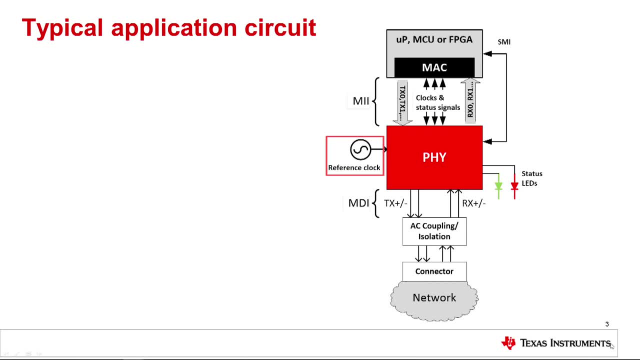 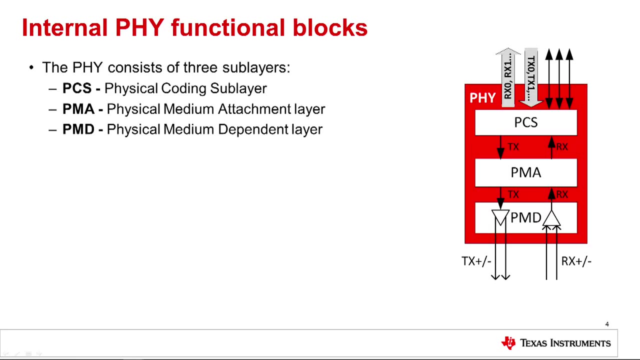 Both of these must meet a minimum frequency accuracy of ±100 ppm, accounting for all error sources. Some of the details on clocking XMII, SMI and MDI will be covered in other Precision Lab sessions. about Ethernet, The IEEE 802.3 standard defines three major functional blocks or sublayers that make up the PHI. 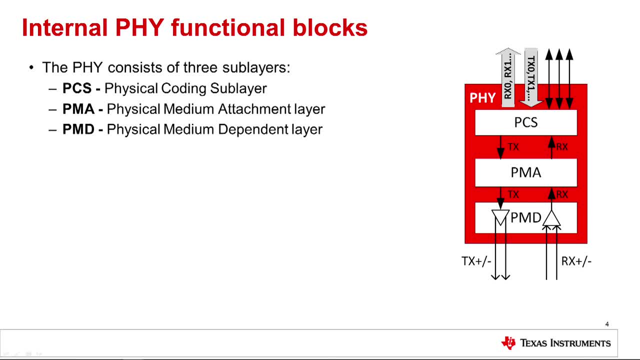 These layers are the physical coding sublayer, or PCS. The primary function of the PCS is to encode and decode data. For example, in a 100Base TX, 4 bits of data received from the MAC interface to be transmitted over the network. 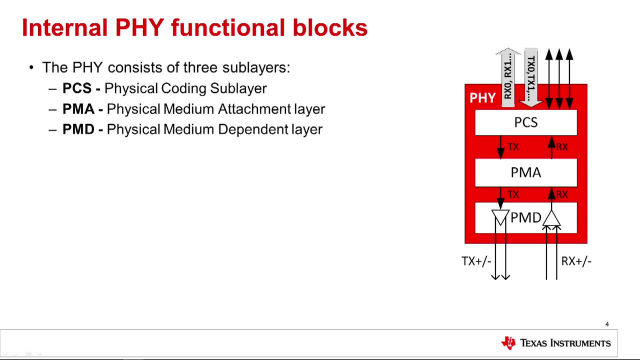 are encoded to a 5-bit block code. Hence the total data rate transmitted over the channel becomes 125 Mbps. The use of block codes helps with clock recovery at the receiver and provides additional codes that are used for link management. The physical medium attachment sublayer, or PMA. 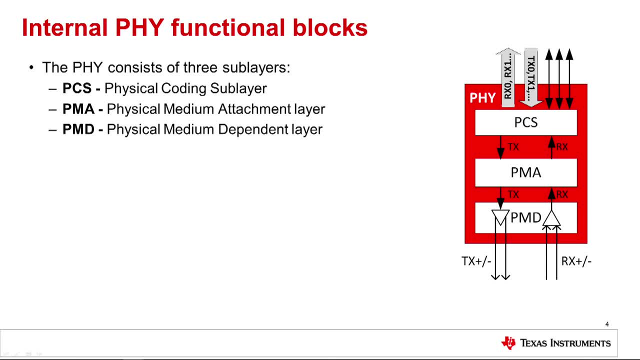 provides functions for bit-to-symbol mapping, determining link status, clock recovery and detecting error events. The physical medium dependent sublayer, or PMD, implements the functions that support the PHI's physical connection to the network, whether it is copper or fiber. 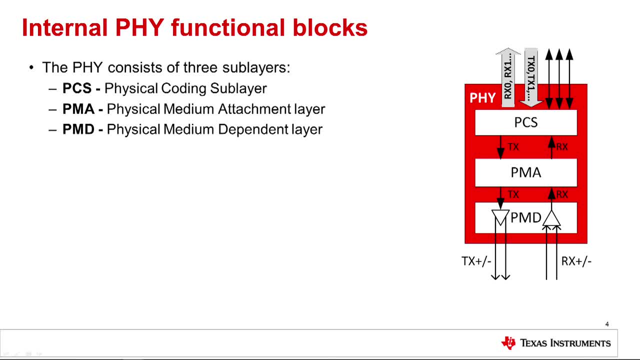 Each layer contains both transmit and receive paths. The PCS block is responsible for receiving data from and transmitting data to the MAC. While the PMA function is always present in the PHI, the PMD may not be. This is determined by the versions of the Ethernet standard supported by the MAC. 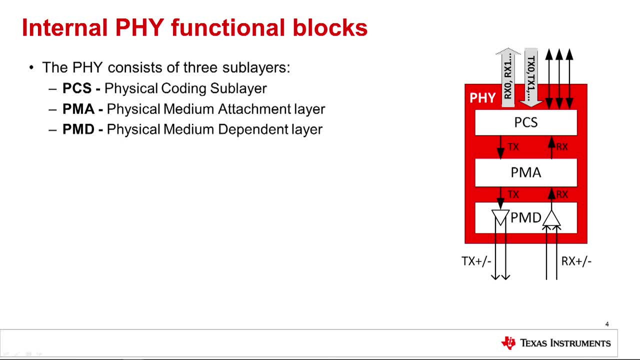 In some versions of the standard, the PMD functions are included in the PMA. Regardless, these blocks are the interface to the physical medium and they provide services that convert electrical or optical signals to bits in the receive path and bits to electrical or optical signals in the transmit path. 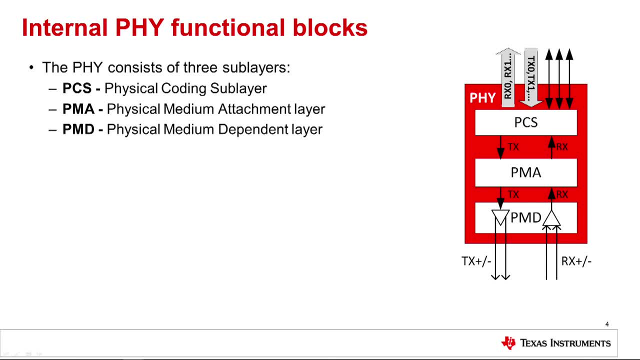 Though the diagram here shows separate transmit and receive channels in the physical medium, the physical medium may actually be shared between RX and TX. In this case, hybrid and echo canceling functions hosted in the PMA PMD allow the PHI to successfully receive data over the link. 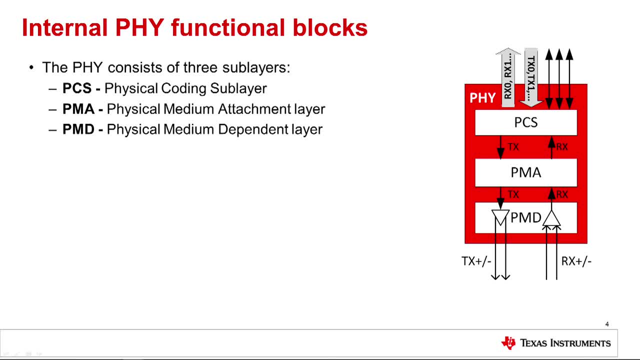 at the same time it is transmitting. Finally, the physical medium may consist of multiple parallel physical channels that enable the transmission and reception of data at higher rates. For example, 1000BaseT uses four twisted pair channels: A, B, C and D. 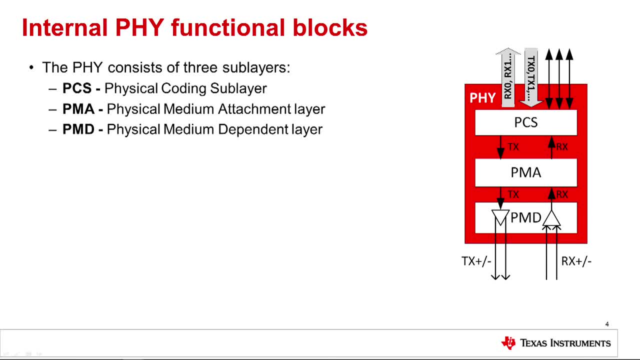 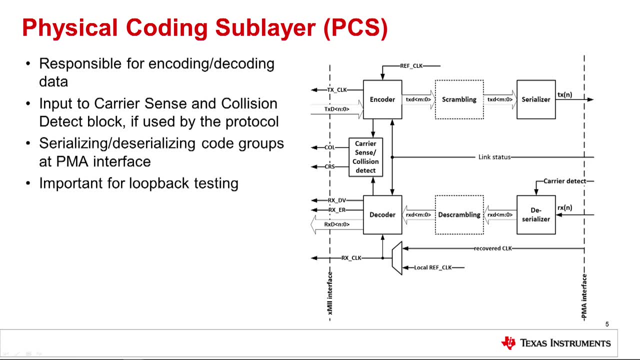 each supporting 250 Mbps to achieve a total data rate of 1 Gbps. The physical coding sublayer, PCS, provides different services to the MAC layer and PMA. It is primarily responsible for encoding and decoding data passed over the link. The PCS exchanges, transmit and receive data. 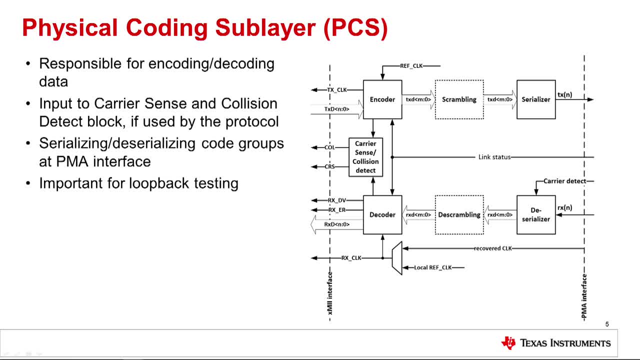 and other control signals from the MAC. The PCS also monitors the MAC layer through the XMII interface. The widths of the transmit and receive data paths between the PHI and the MAC, here labeled as TXD and RXD, may have values of 1,, 2,, 4, or 8 bits. 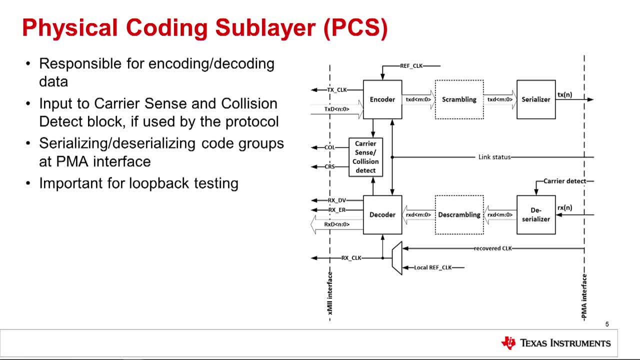 depending on the total data speed. The PCS also contains functions that monitor both the transmit and receive paths to determine when the network interface is active and if there are collisions. signal the MAC layer- the occurrence of a collision using the COL signal. It supports low power mode if implemented. 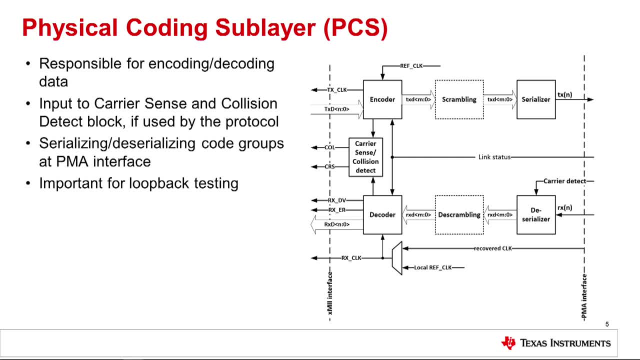 by processing idle code groups. The receive path of the PCS takes in data from the PMA interface and basically reverses the processing that the PCS and the sending node apply to the data. It decodes the receive code groups to the original packet bits. 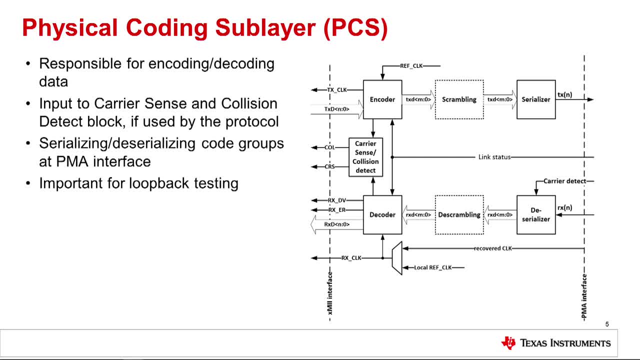 Based on either the success or failure of proper data decode and recovery. the receive block will either assert an RXDV signal to indicate it is forwarding valid data to the MAC or a certain RXER signal to indicate it has detected an error in the data. 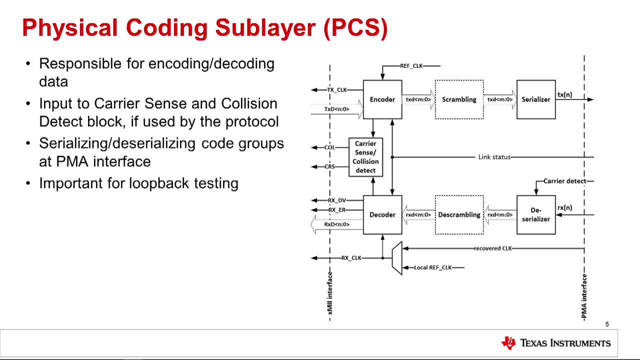 The PHYS clock recovery function is used to synchronize its receiver bit clock to the transmitting PHYS bit clock. This is vital to understand when performing loopback testing. If all is decoded and encoded properly, the same number of receive and transmit packets should be the same with no errors. 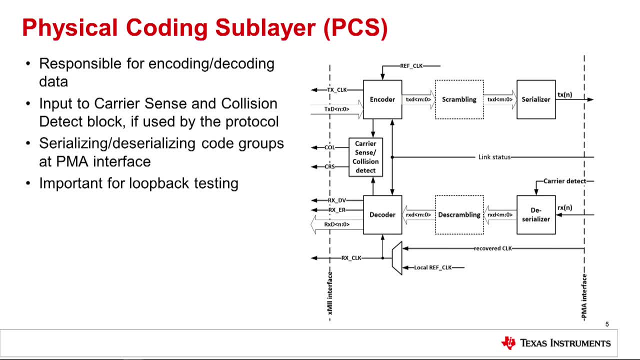 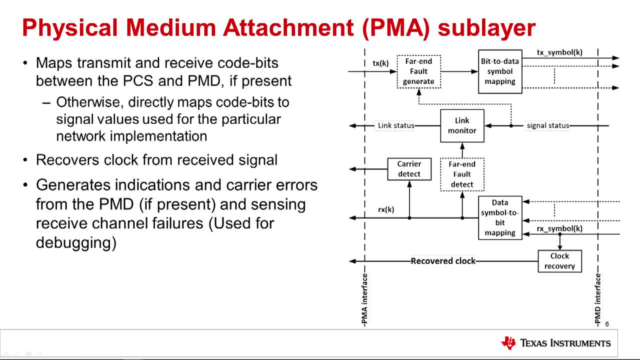 In some versions of IEEE 802.3 standard, additional scrambling is applied to the data. The main function of the physical medium attachment sublayer, or PMA, is to convert the encoded transmit bit stream from the PCS sublayer to the appropriate data symbol. 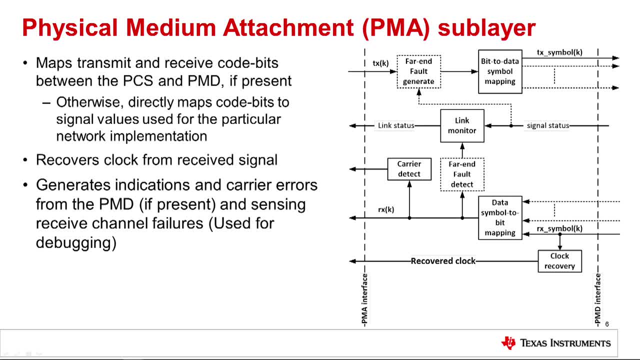 for transmission on the network medium and convert incoming data symbols from the network into bits that are then passed to the PCS sublayer. The PMA sublayer also performs carrier detection by looking for a link transition from the idle state in the received bit stream: RXK. 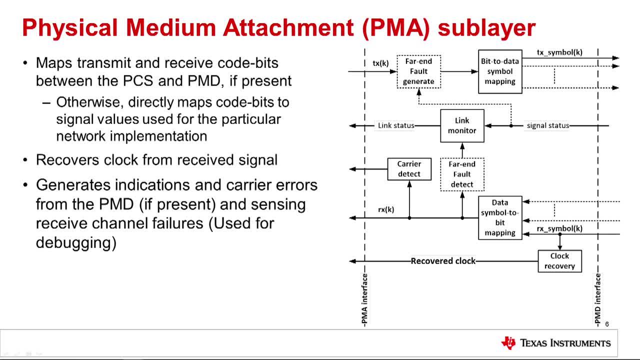 When this transition is detected, it then looks for the start of stream delimiter SSD. Once the latter is detected, it indicates carrier detection to the PCS sublayer. It also monitors the signal status reported by the PMD sublayer, if present. If the auto-negotiation capability 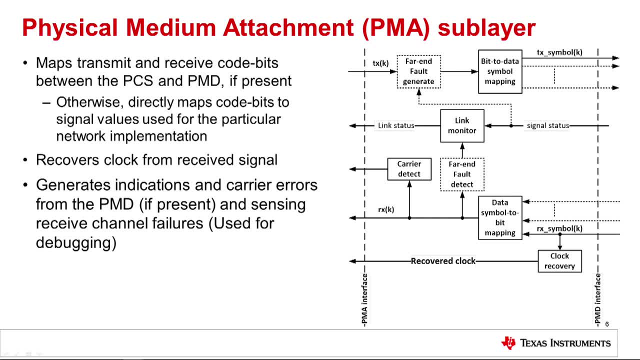 has been implemented in the PHI, the PMA sublayer will coordinate with the latter and set the link status indication to the appropriate value pending the state of auto-negotiation, and pass this to the PCS. Otherwise, it sets the link status according to the signal status. 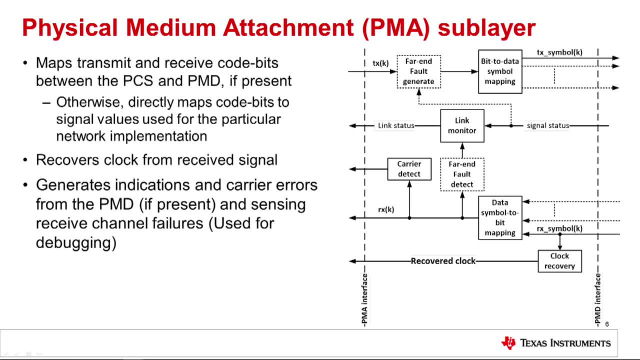 indicated by the PMD. If the PHI does not support auto-negotiation, it may instead include an optional far-end fault detect capability. If the PHI detects a physical error condition in the received channel, it will generate a fault indication and insert this in the TX channel stream. 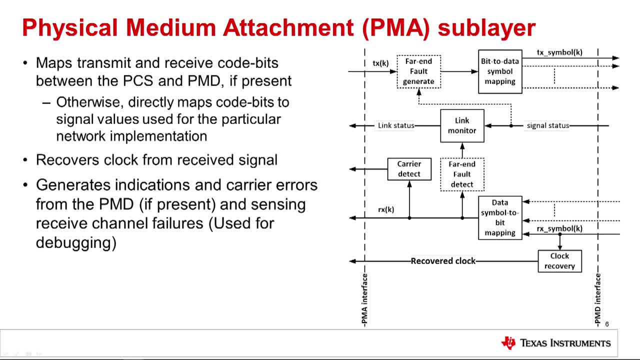 If it receives a far-end fault indication in the RX channel, which is a special symbol pattern, it will begin transmitting an idle symbol pattern to insist with re-establish of normal communications. Note that far-end fault detect is not supported if the PHI is capable of auto-negotiation. 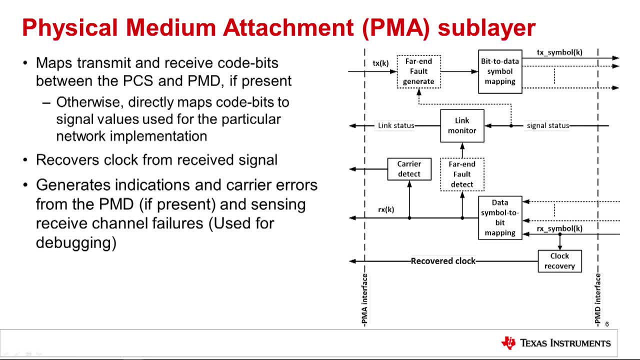 Some optional functionality that the PMA performs also include generating indications and carrier errors from the PMD, if present, and sensing received channel failures, then transmitting or detecting far-end fault indication. This is useful for any debugging on the PHI: Proper functioning of the PMA. 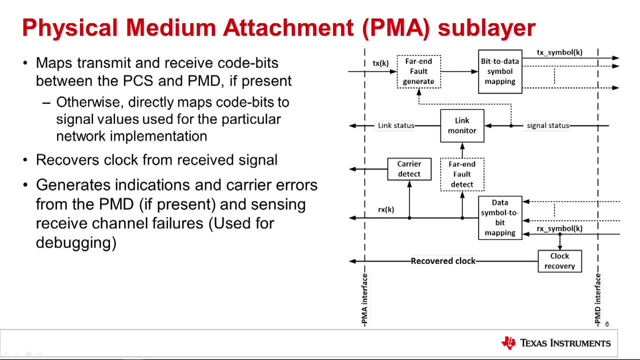 is important as it needs to pass compliance tests. Finally, note that for versions of the standard that use multiple twisted pairs, such as 1000 base T, there will be no problem with one-to-n mapping of the symbol stream, For example, 1000 base T. 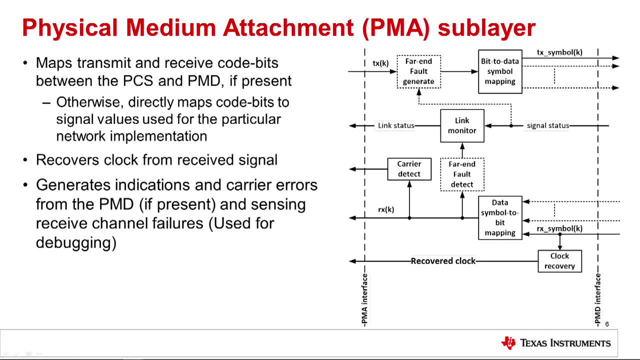 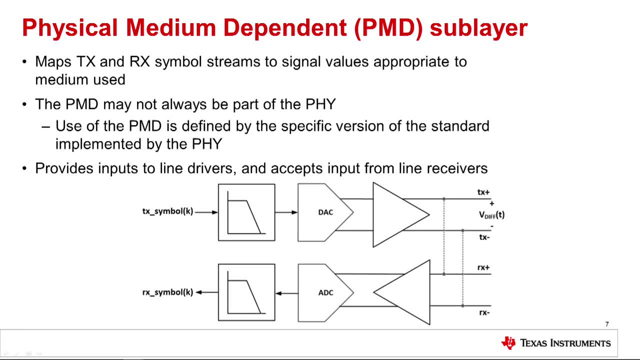 uses four twisted pairs designated as channels A, B, C and D. The physical medium dependent symbol layer, or PMD, if implemented in the PHI, is primarily responsible for converting the TX symbols to the appropriate physical signals used for the network medium. It also converts the received path signals. 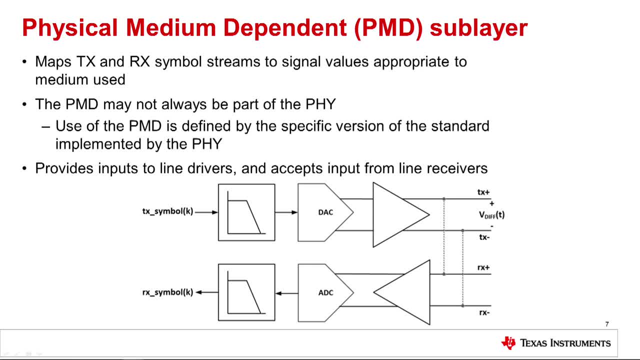 to RX symbols in the received path. The PMD may not always be part of the PHI. The use of the PMD is defined by the specific version of the standard implemented by the PHI. The standard defines systems that accommodate certain mediums and types of cabling. 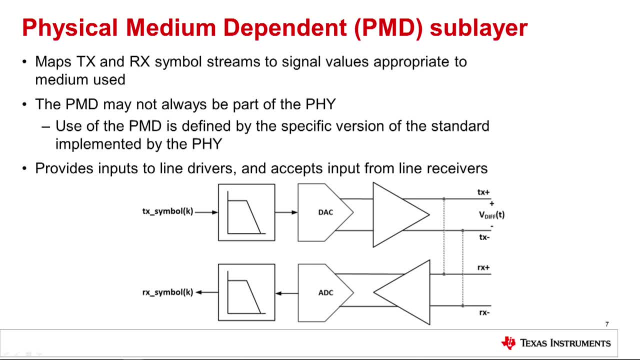 In some amendments to IEEE 802.3 standard, for example IEEE 802.3 BW, which is also called 100 base T1, the PMD is not defined because only single twisted pair copper is supported. In this case, the PMA handles the task of conversion. 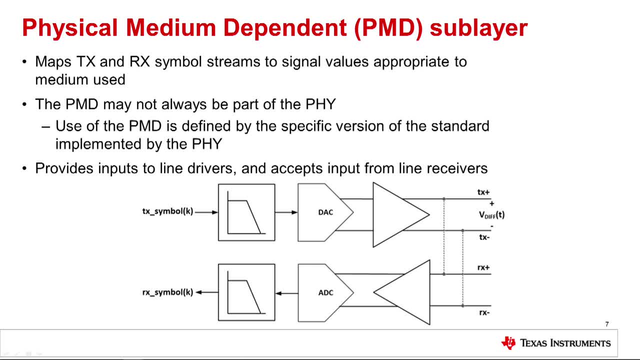 between symbols and signaling. This is also true for 1000 base T. 1000 base TX defines PMD functionality, but 1000 base T does not. The PMD is useful for debugging the medium, as it is the physical layer responsible for interfacing. 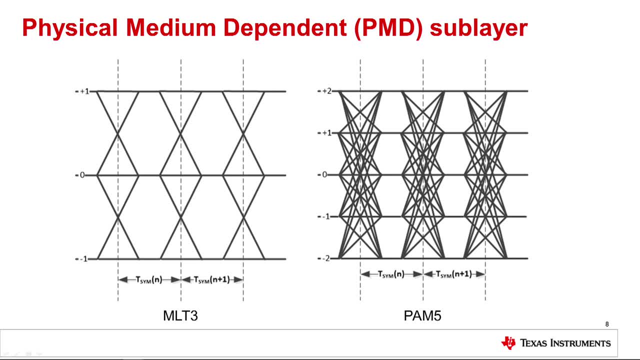 to the physical media, Considering the only network interfaces that use twisted pair copper. for the moment, the electrical format of the signaling is differential. Some examples of the types of signaling used include 100 base TX using MLT3. 1000 base T using PAM5. 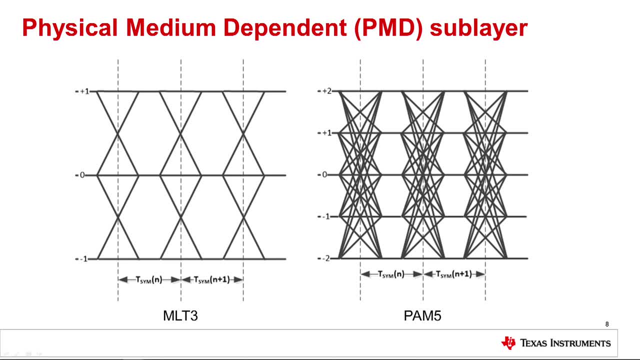 and 100 base T1. Examples of MLT3 and PAM5 are shown here as ideal signals. The symbol values illustrated here are relative values, not actual voltage levels, which are defined in the respective IEEE 802.3 amendments. The actual voltages are also: 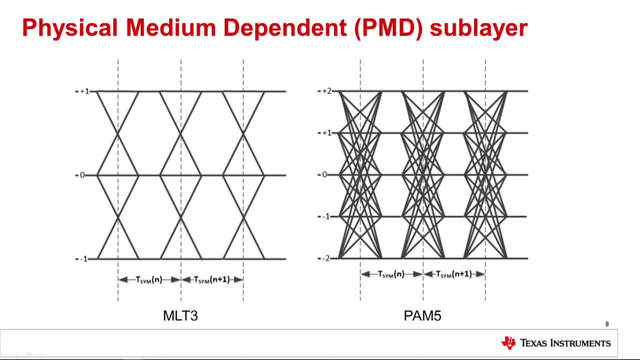 a differential value. For example, Vdif of T is equal to TX positive minus TX negative. More information and details on the different types of signaling will be explained in future videos. For example, the differential signals are usually driven into a twisted pair: differential impedance.